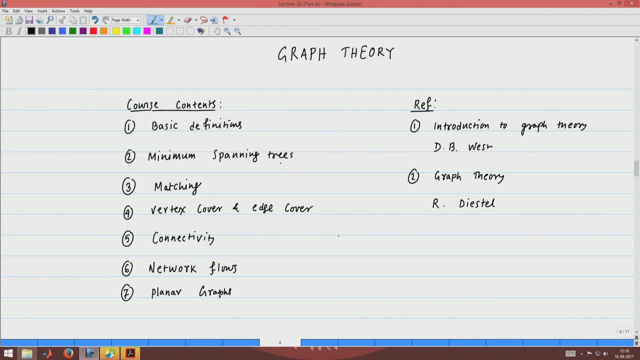 and Kruskal algorithm to find minimum spanning tree in a weighted graph. Third, we talk about matching and we learn how to find maximum matching in bipartite graph. In the fourth module we learn what is vertex cover And we will talk about the vertical curve and 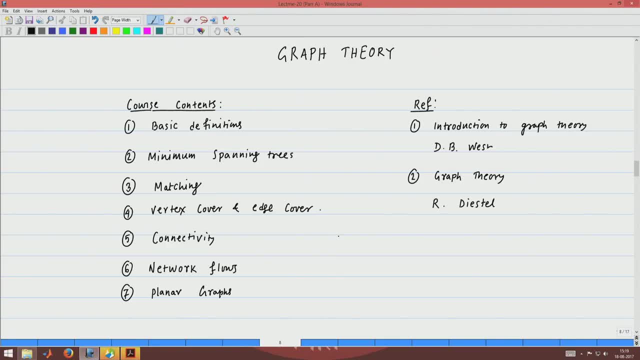 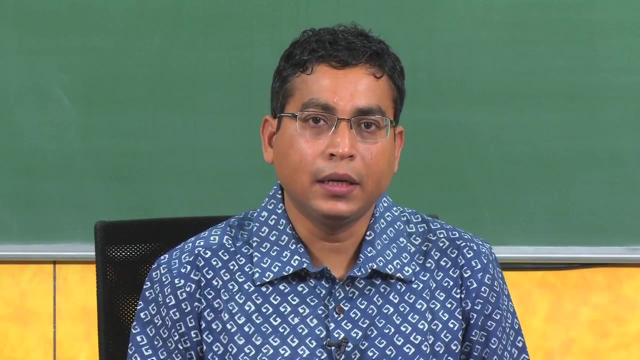 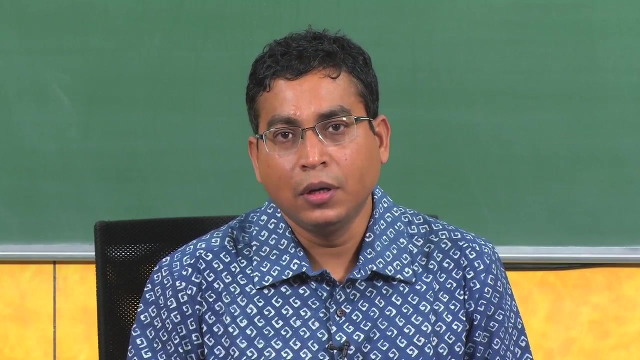 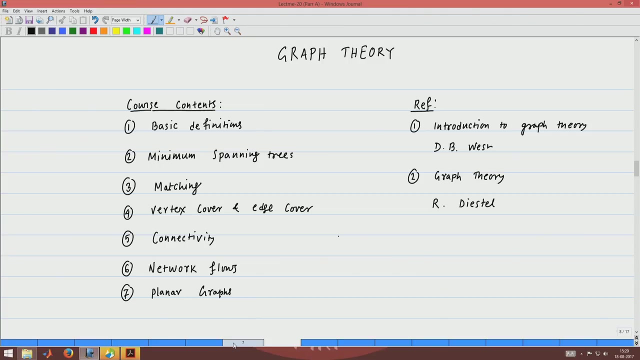 edge cover and also independent set. In the fifth module we will learn what is connectivity. We talk about vertex connectivity of a graph and edge connectivity of a graph and how vertex connectivity and edge connectivity are related. Thank you for your attention. Next we talk about network flows and in this module we learn how to find maximum flow in 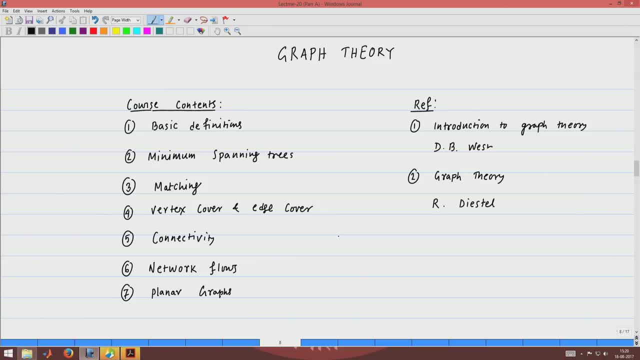 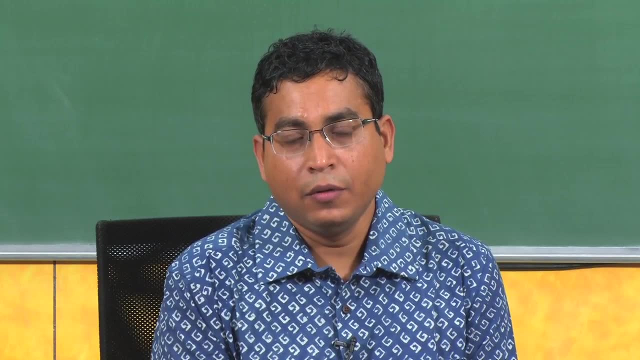 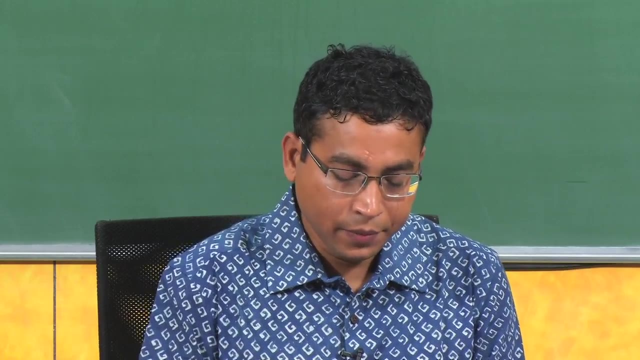 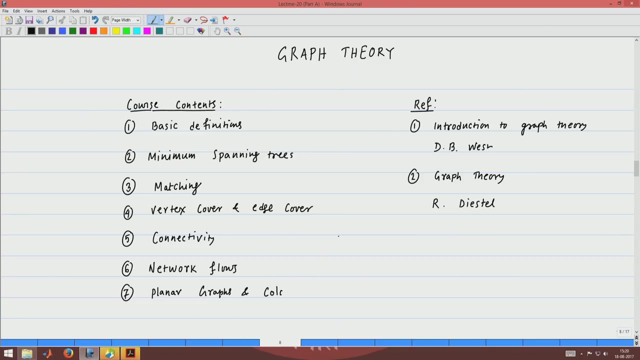 a given network using Ford-Fulkerson algorithm Also, we learn what is minimum cut and we will prove that the maximum flow is equal to the minimum cut. and finally, we talk about planar graphs and graph colouring. So we talk about vertex colouring, edge colouring and colouring planar graphs. 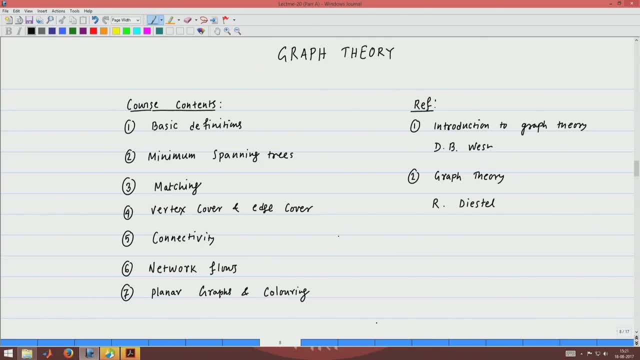 So the reference for this course is Introduction to Graph Theory by DB West and the second reference is Graph Theory by RD Estill. Let me start with the definition of graph. So a graph is a graph where a number of sets appear. 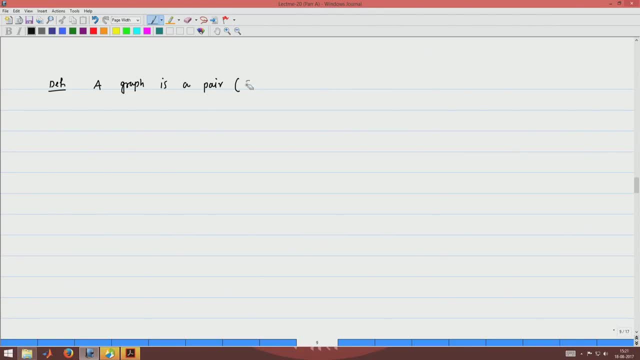 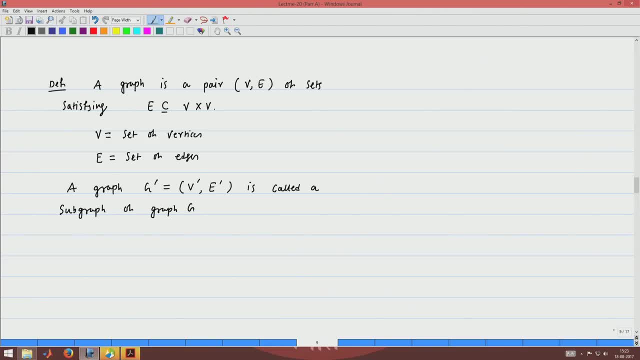 of graph G, if V prime is a subset of V and E prime is a subset of E. So let me give an example of a graph. So these are the vertices of the graph And I call them V1,, V2,, V3,, V4,, V5.. And I call 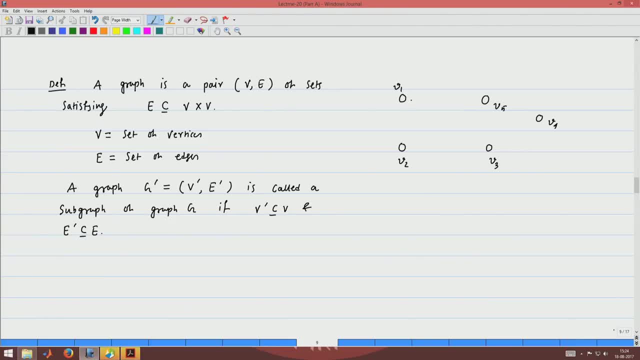 them V1. And edge joins two vertices. So this edge I call E1, which joins V1 and V2.. This is another edge which joins V1 and V2.. I call it E2.. E3 joins V1 and V5, E3 joins V2, V3, E5 joins V2, V3, E3 joins V2, V3, E3 joins V3, E5 joins. 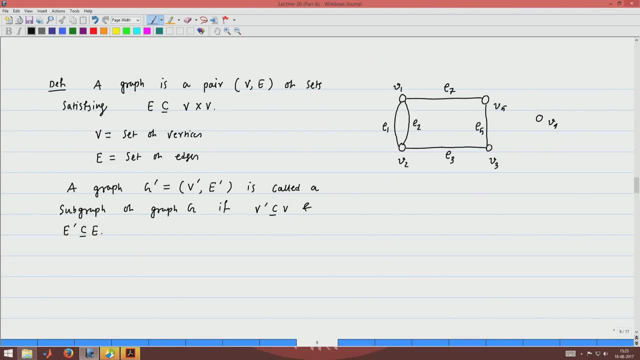 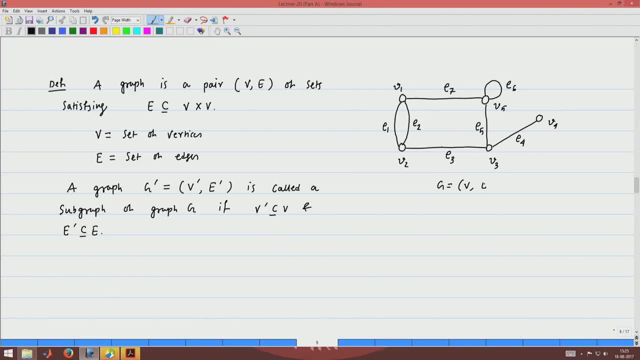 V3, V3, V4, V5, and the edge set consists of E1, E2 up to E7.. If there is an edge joining Vi, V3, V3, V4, V5,, V3, V3, V4, V5, and the edge set consists: 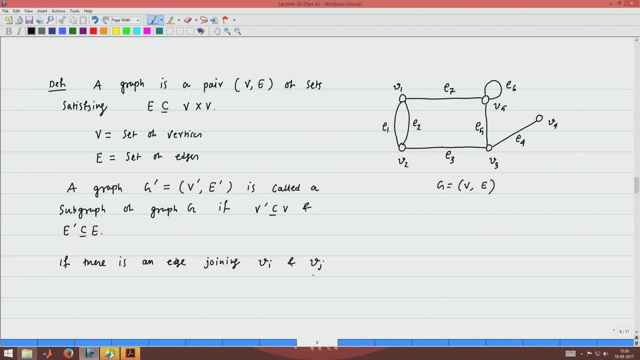 of E1, E2 up to E7. If there is an edge joining Vi and Vj, then they are adjacent. So here you can see that V2 and V3 are adjacent because they are joined by an edge- E3- whereas V2 and V5 are not adjacent. 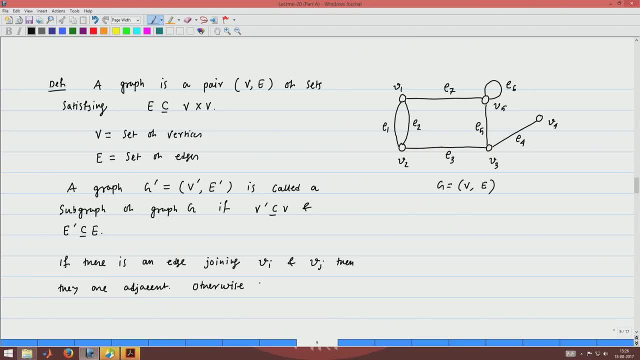 They are non-adjacent. Two or more edges with the same edge set are non-adjacent because they are non-adjacent. Okay, Okay, Okay, Okay, Okay, Okay. So these two end points are called parallel edges and a graph is simple. 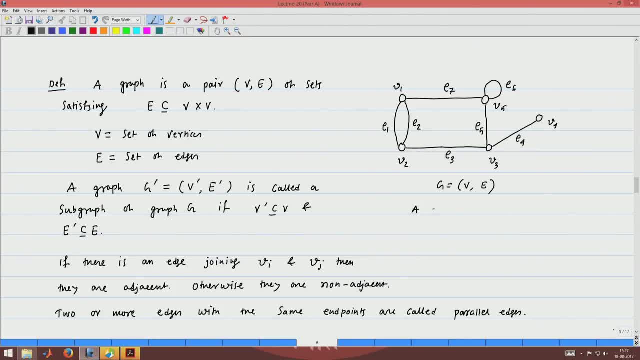 Okay, Okay, Okay is simple: if it has no loops for parallel edges. So for example, here E1 and E2 are parallel edges and E6, so E6 is a loop, E6 is a loop, Whereas E1 and E2 they are parallel edges because they have the same end points. 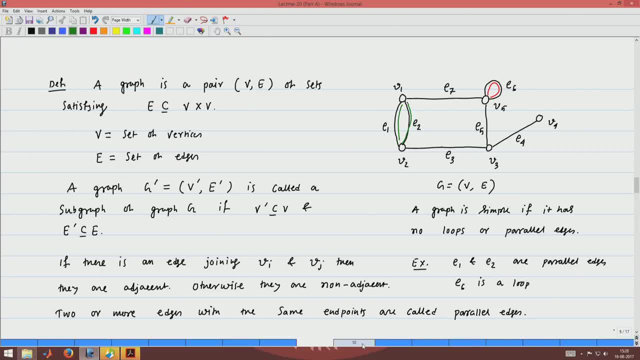 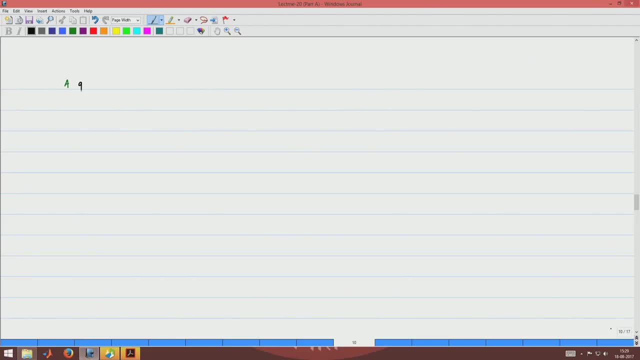 So next we talk about complete graph. A graph is complete if every pair of vertices are adjacent. So, for example, this is a complete graph with one vertex that is called K1, so this is a complete graph with K2.. Okay, So this is a complete graph with two vertices. this is denoted by K2.. 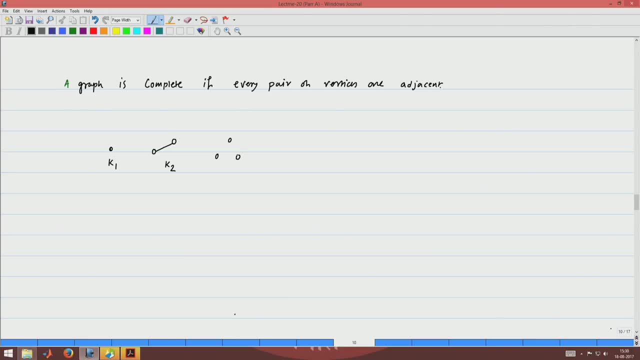 This is a complete graph with three vertices. this is called K3.. This is a complete graph with four vertices: K4.. Okay, Okay, So a complete graph with n vertices is denoted by Kn. Okay, Okay, So definitely, the number of edges of a complete graph with n vertices is the number of edges. 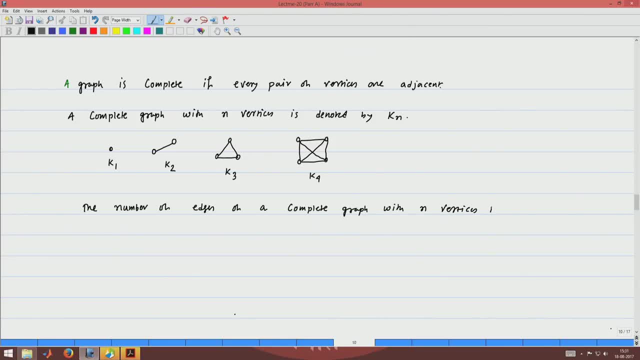 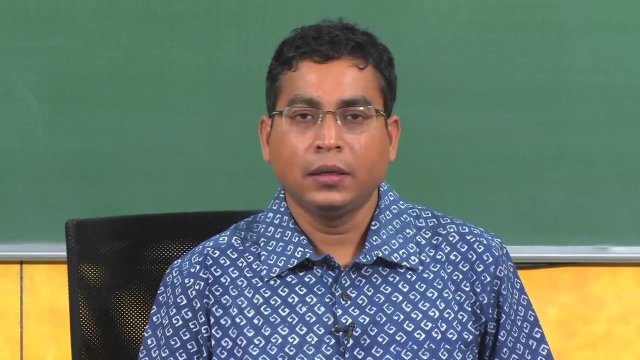 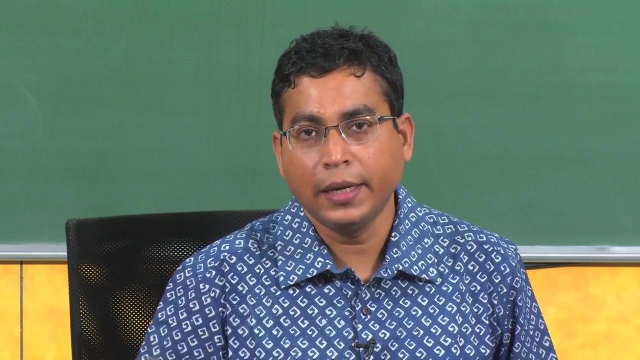 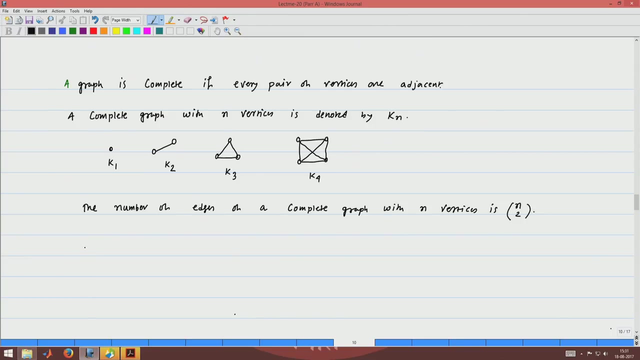 Okay. Okay is n choose 2, because if there are n vertices, then every pair of vertices are joined by an edge. So there will be n choose 2 pairs and n choose 2 edges. Next, a graph is finite if both the number of vertices is the cardinality of V and cardinality. 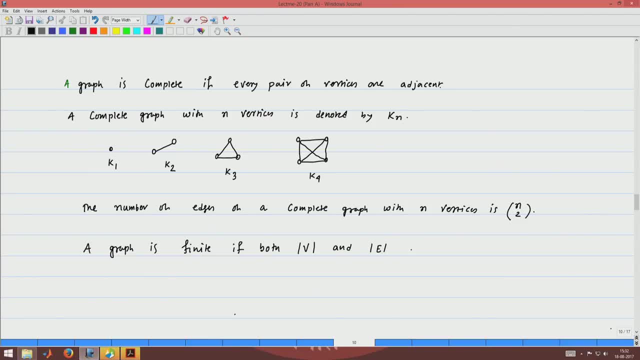 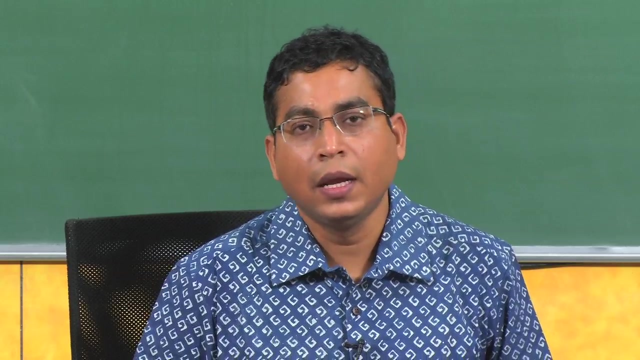 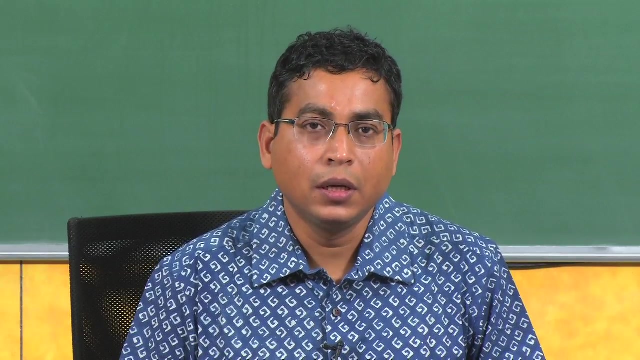 of E are finite and a graph is infinite, So if cardinality of V or cardinality of E is infinite, So we understand a special type of graph now that is called complete graph And kn is the notation for complete graph with n vertices. 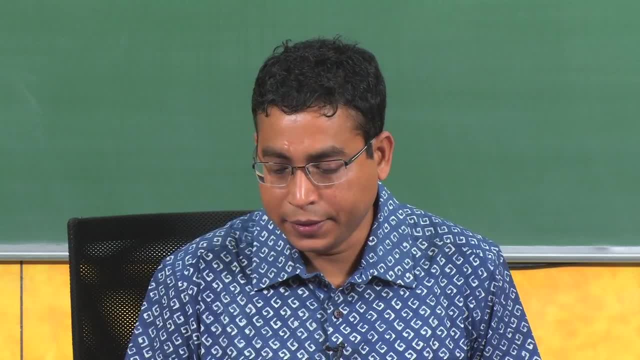 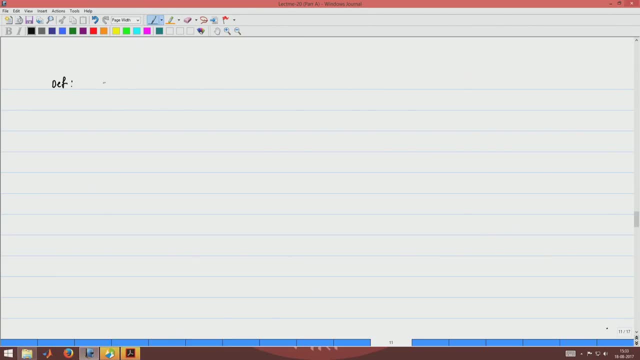 Now. next we will learn what is degree of a vertex. definition: The degree of a vertex: okay. Number of vertices: okay. V in a graph G, denoted by dV, is the number of vertices. Now we will learn the fundamental number of vertices. 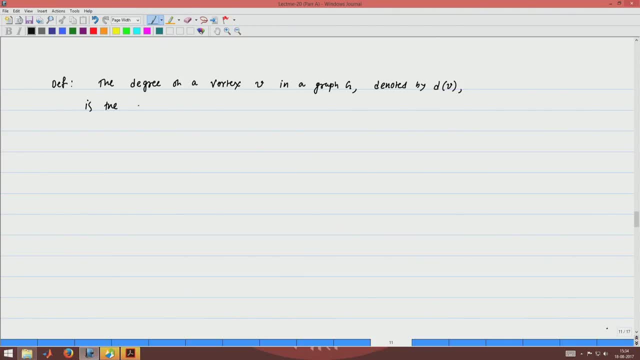 D is the number of vertices. Okay, Here you do not have to think about that Right number of edges of G incident to V. okay, So let me give an example of a graph. So I label these vertices by V1,, V2,, V3,, V4, and there is a loop here. 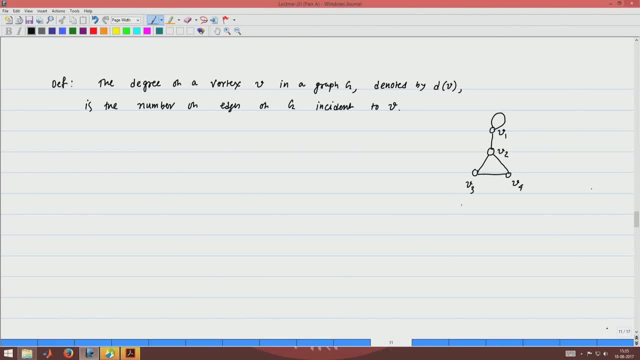 So here you can see that the degree of degree of V3 is equal to 2 because 2 edges are incident to V3, degree of V4 is also 2 because there are 2 edges incident to V4.. Degree of V2 is equal to 3 because there are 3 edges incident to V2 and the degree of V1. 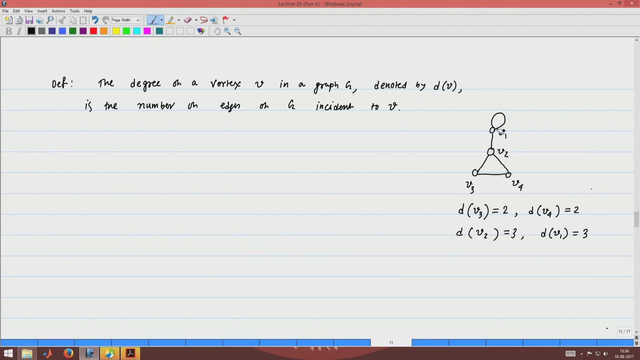 is also 3, because this will be counted 2 degree plus 1 degree. here A graph G is said to be K regular. if the degree of V is equal to K for all vertices, V belongs to K. okay, So an example of a regular graph. this is called C4, cycle of length 4. you will learn soon. 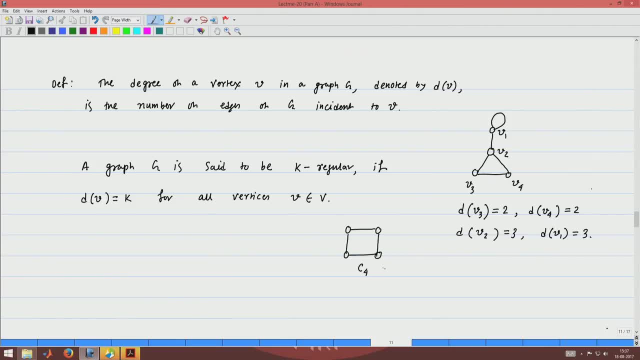 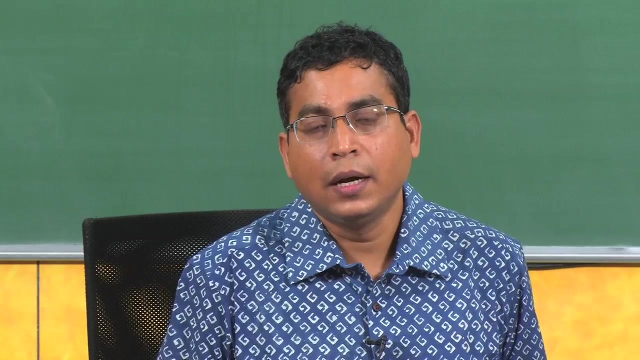 1. can see that the degree of every vertex is 2, so this is 2 regular graph. okay, and one observation: that a complete graph on N vertices is N-1. okay, So this is because a complete graph with N vertices, every vertex is adjacent to all the. 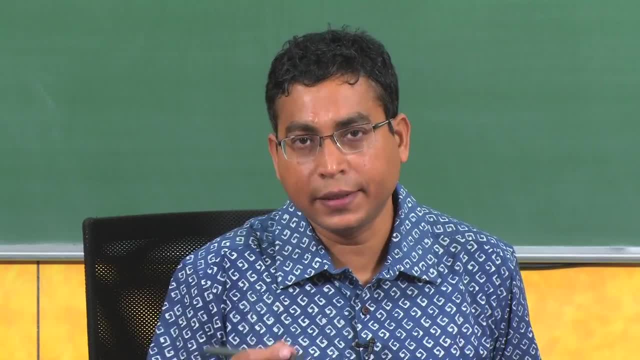 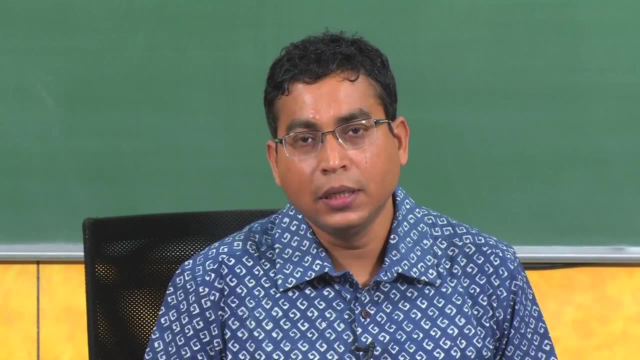 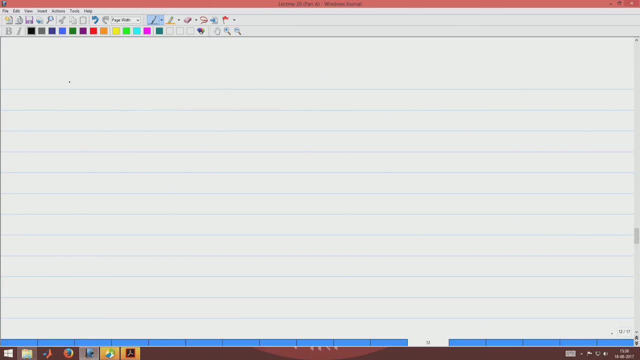 remaining N-1 vertices, so every vertex is having degree N-1, so a complete graph with N vertices is N-1.. Next we will talk about a theorem. if a graph G with E adjacent- Okay Okay, Okay. So if a graph G with E adjacent has vertices V1, V2, Vn, then the degree sum, degree of 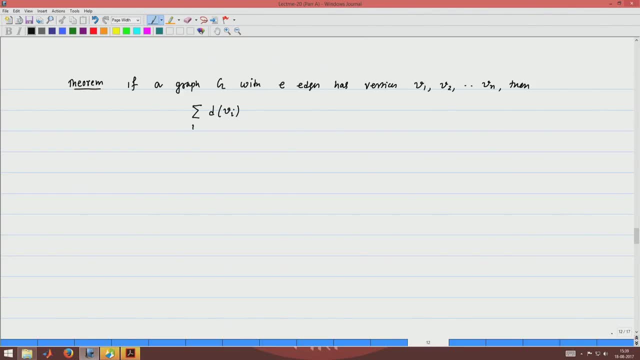 the vertex Vi. Okay, I, equal to 1 to N is equal to twice the number of edges. So E stands for the number of edges and N stands for the number of vertices. So in our previous example, if I see that here, the number of vertices is equal to twice the. 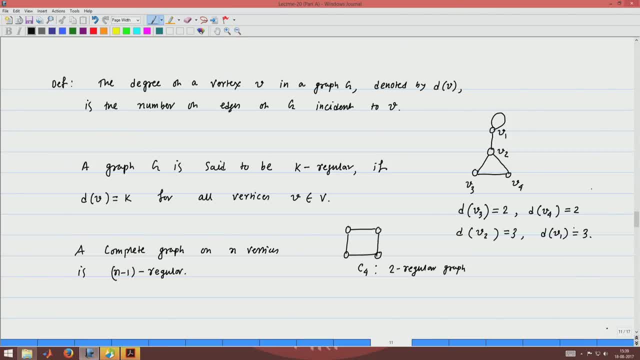 number of edges. Okay, So the degree sum? there are 4 vertices. the degree sum is summation of dM of Vi from 1 to 4 is equal to 10, and this graph has 5 edges, so E equal to 5.. 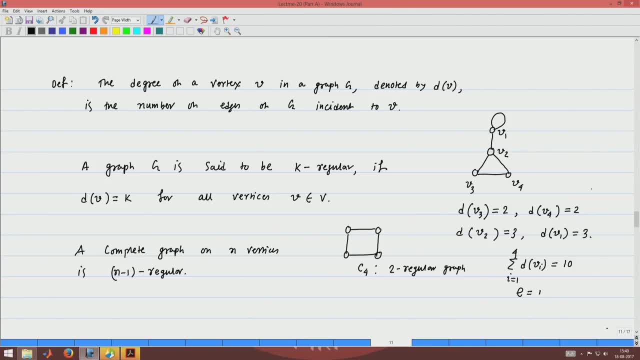 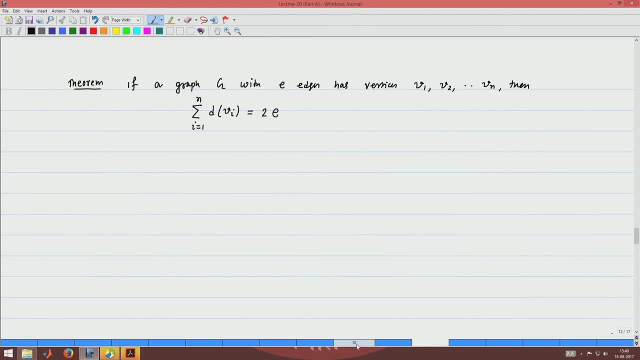 So this degree sum is equal to 10.. Yeah, Okay, So this degree sum is equal to twice of E, right? So it is an easy observation, because the proof is that every edge contributes to in the degree sum. That is why this is the degree sum is equal to n. So you can see here that this edge 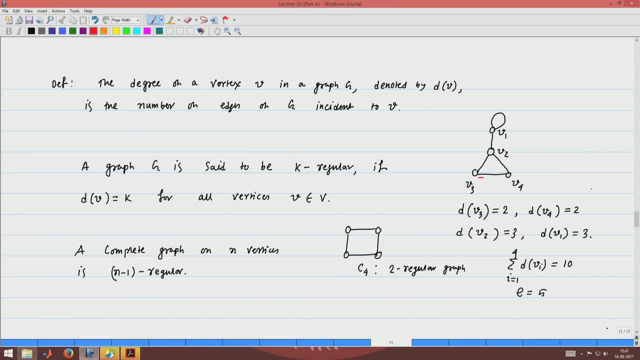 for example, this is contributing 2 degree in the degree sum, So 1 degree is counted as degree of V4.. Degree of V4 is 2 because of this edge And this edge, and the degree of V3 is also 2 because of this edge and this edge. So 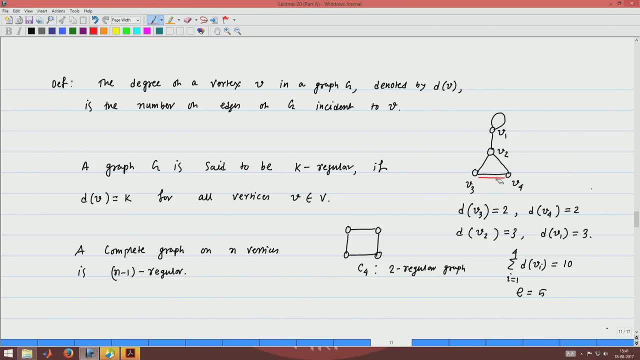 this edge is contributing 2 in the degree sum. That is why the degree sum is twice the number of edges. Now we denote something called maximum degree, So that this notation, that delta of g, is equal to the maximum degree. So we will use this notation several times. 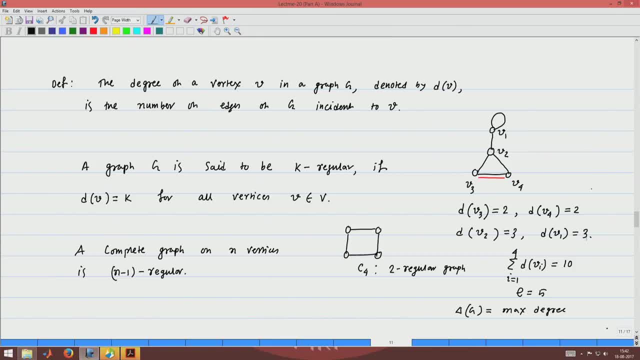 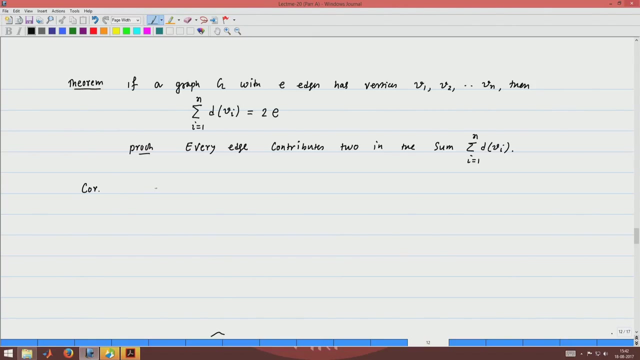 and the maximum degree here is 3.. So this is 3 here, and small delta g is the notation for minimum degree and the minimum degree here is 2. right Now the corollary of this theorem in a graph G: 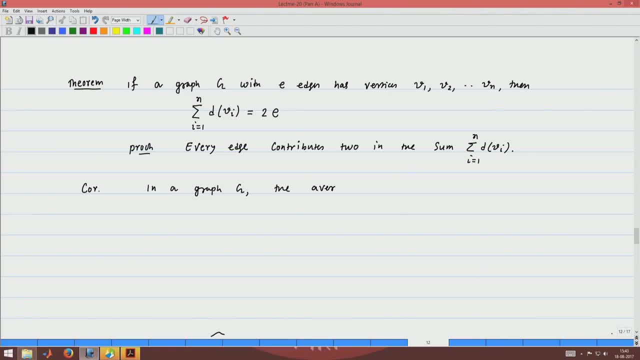 is twice e by n, because this is the degree sum and there are n vertices. so that is average degree of every vertex is twice e by n and obviously this average degree twice e by n, it will be smaller than the maximum degree and this will be the average degree will be. 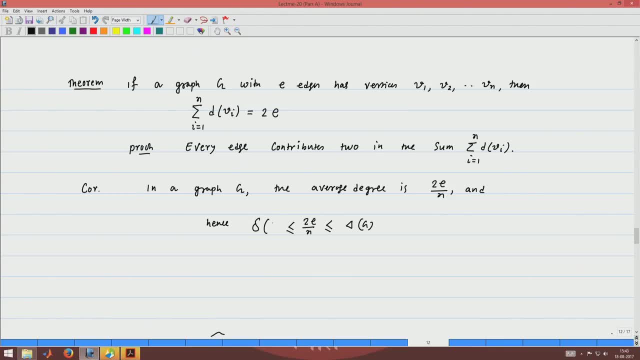 greater than the minimum degree of the graph G. Okay, so these are all fine. next we talk about another theorem. This says that in any graph G, the number of vertices with odd degree is even. So if I draw this graph again now, this vertex has degree 2, this vertex has degree 2, this. 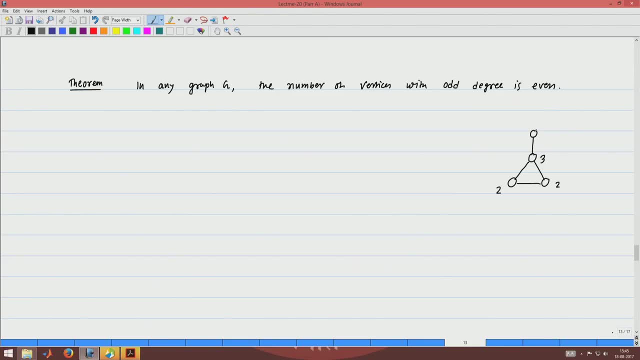 vertex has degree 3,. this vertex has degree 3.. Now you can see that the number of vertices having odd degree is 2, and that is always true. Why this is true? Here is the proof of this. Let V1, V2 and Vn be vertices of G and for. 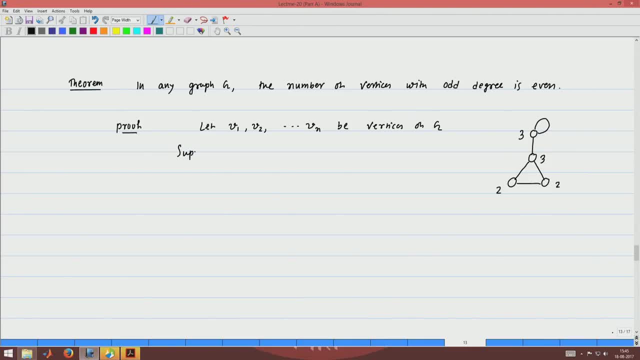 simplicity suppose. Now what we know is that the degree v t plus 1 plus the degree of v n, that is the degree sum, is equal to twice a. Now what? 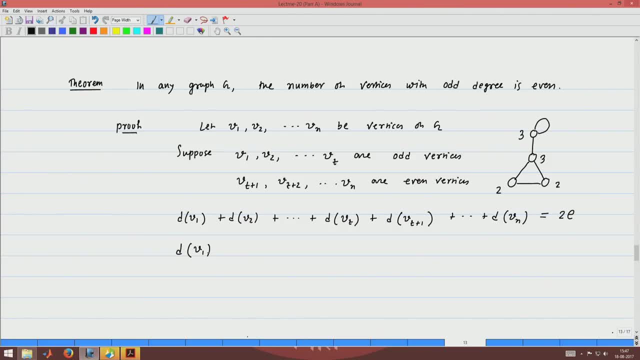 we can do is that I can write degree of v 1 plus degree of v t. these are the odd vertices, So equal to twice e minus degree of v t plus 1 plus degree of v n. Now this is 2, e is: 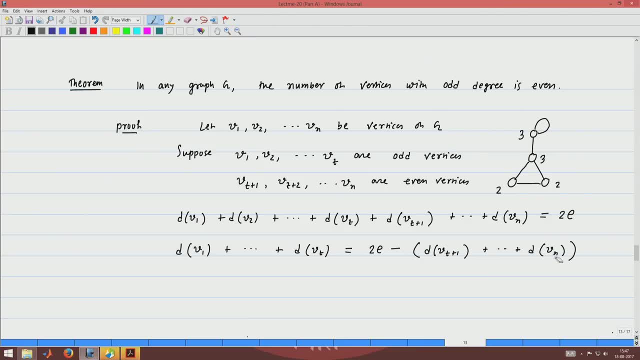 even, and these are all even vertices. So this is also even So. this is even So the whole thing. the right hand side is even. the whole thing is even minus, even So, it is even now. we know that this each term here.